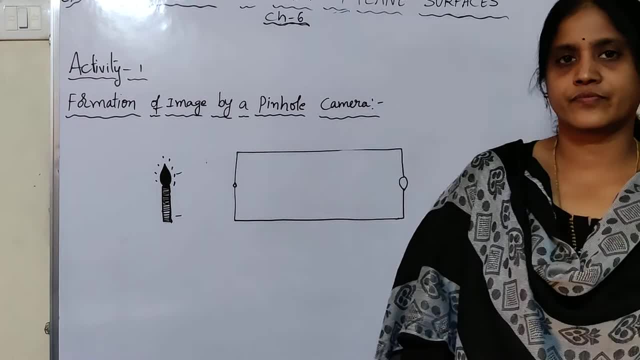 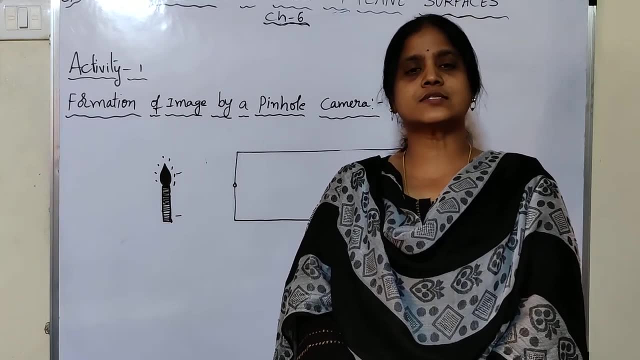 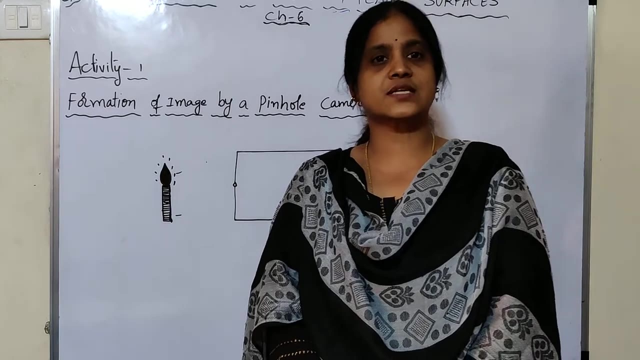 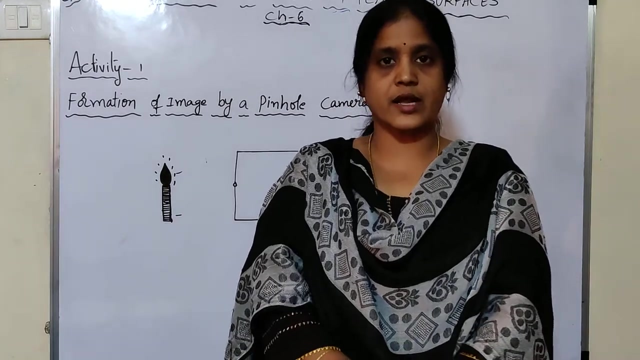 Good morning students. Welcome back to the session. In previous video we have discussed about some important terms which are related to reflection of light. So what are the terms? we discuss Types of objects, based on the concept of when light falls on any object. 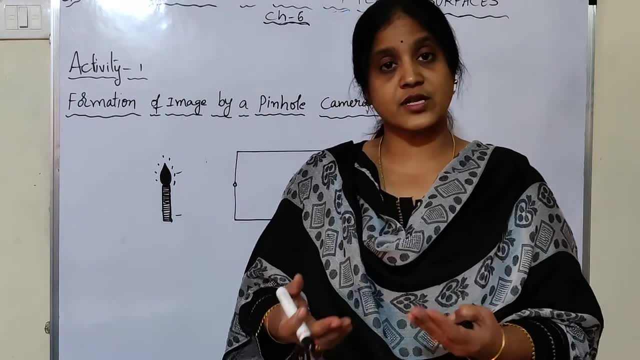 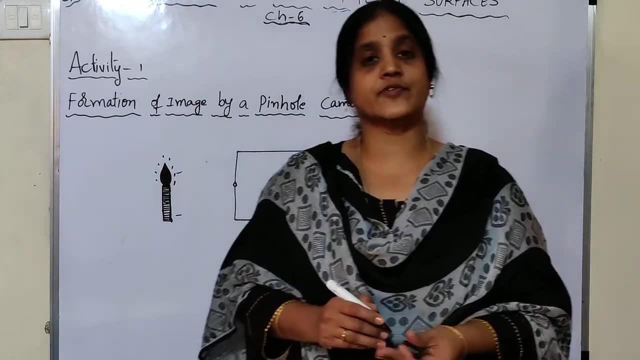 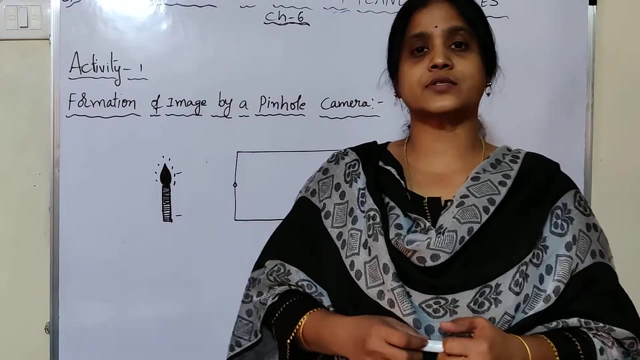 whether the object absorbs the light or otherwise, whether the object allows the light rays to pass through them or not. Based on that, these objects are classified into three types. What are that? Transparent objects, translucent object and opaque objects. And one more point. 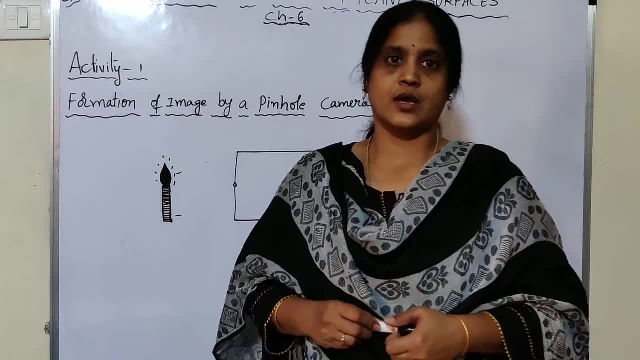 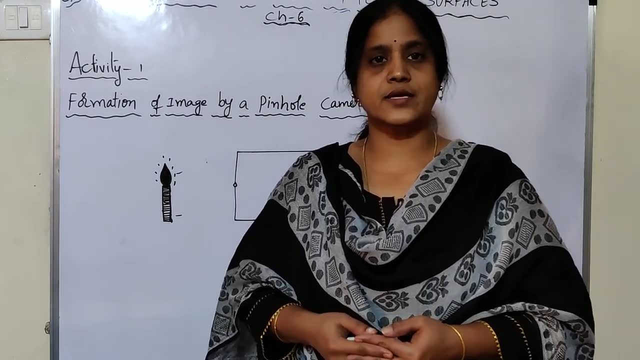 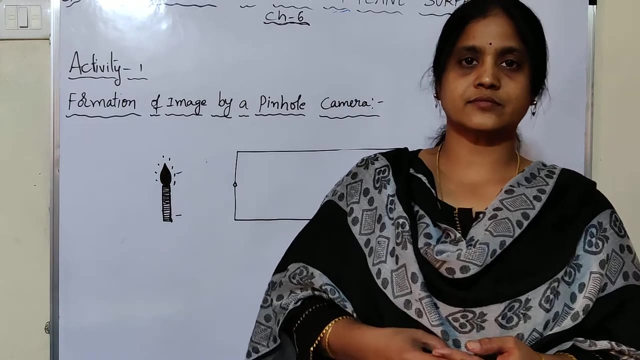 light, the rectilinear propagation of light. What is rectilinear propagation of light? Light always travels in stripes, And the last one is sorry. one more point is for the formation of a shadow. what are the materials required? This is one more question, important question Once again: what are the? 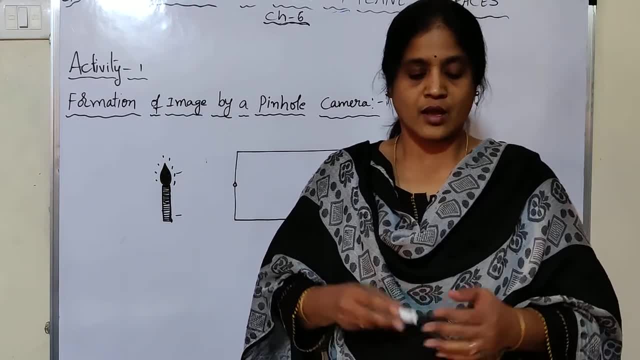 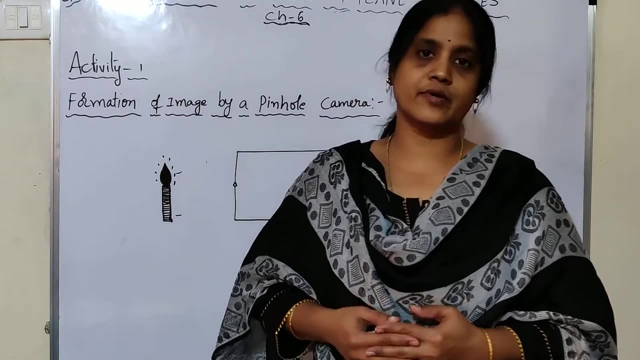 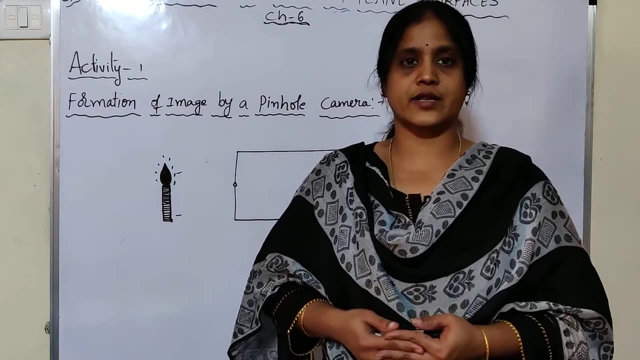 materials required for the formation of a shadow, An opaque object, source of light and screen. And the last point is loss of reflection. Now, in this video, we will discuss about the three types of objects based on the concept of light. We will discuss about different activities or otherwise activity wise, which. 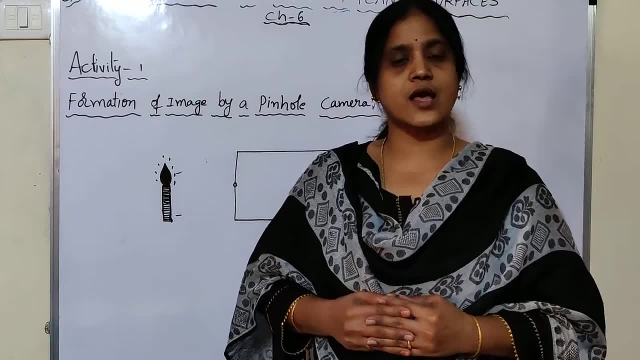 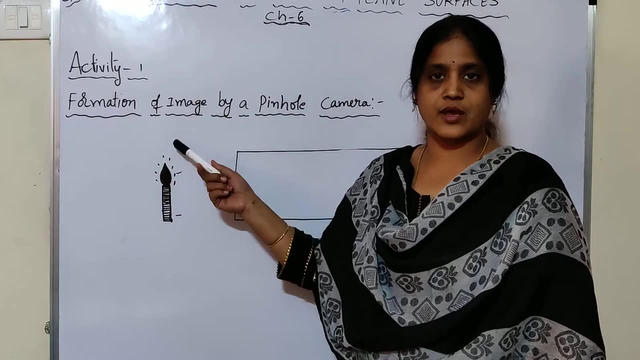 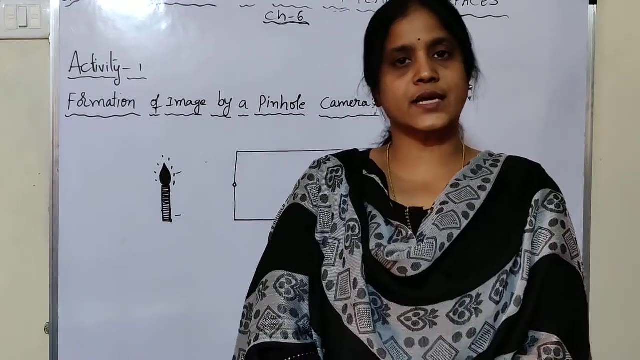 are given in our textbook. So let's start with activity one. What is that Here? activity one: formation of image by a pinhole camera. First, what is a pinhole camera? What is a pinhole camera? See, children, you know about this pinhole camera in earlier classes in. 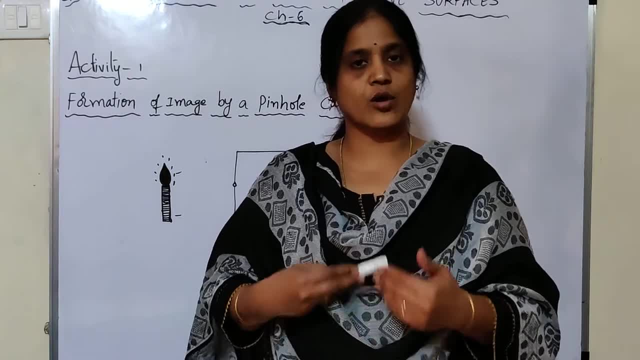 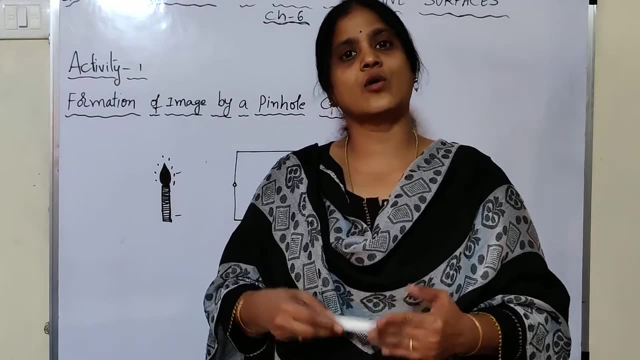 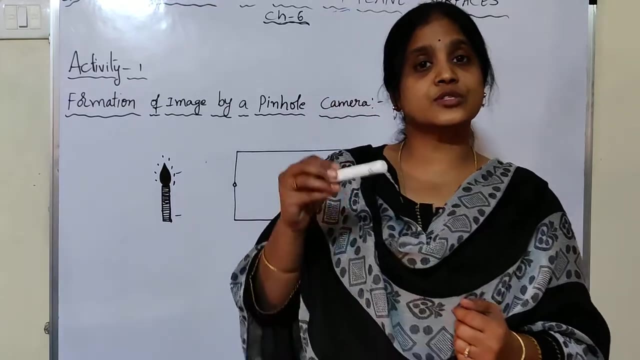 class 8th and 7th. So once we will recall the points which are related to the pinhole camera- how does it works, based on which principle it works, and how to prepare this pinhole camera- and we will discuss and we will learn in 8th class how to draw a rediagram. 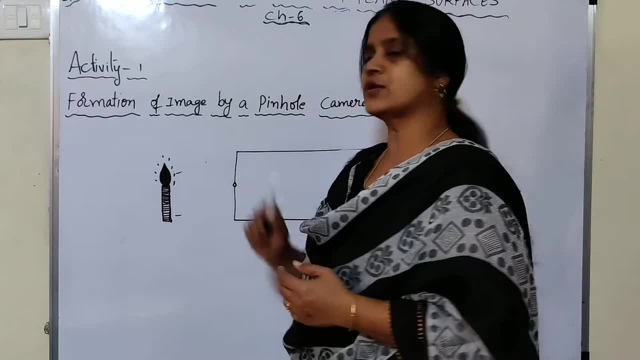 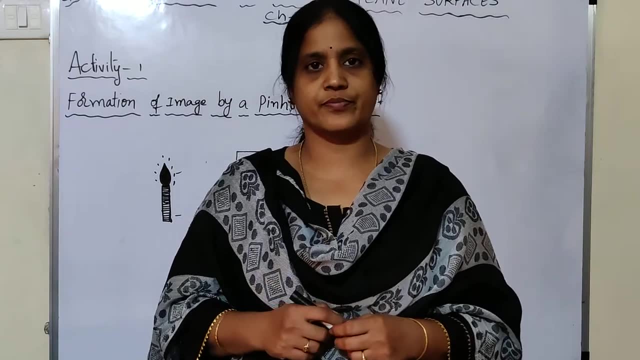 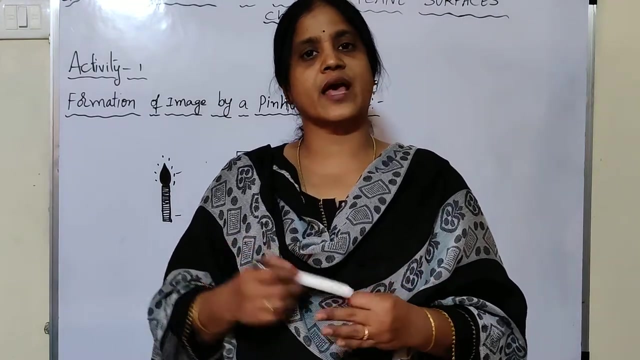 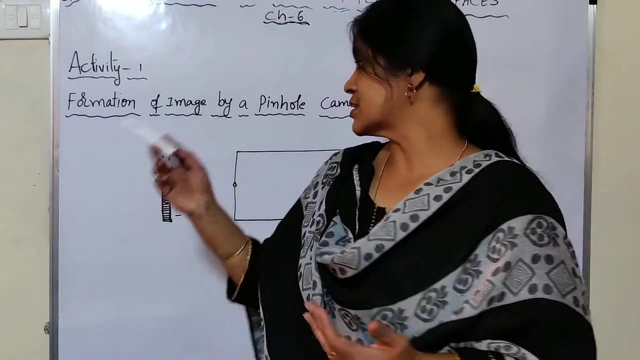 for the formation of image by a pinhole camera. Actually, this pinhole camera is a simple kind of camera. we have a simple kind of camera and it does not have a lens. generally in cell phones and cameras we use lenses. by using the lenses we can take the photos and all we can get. but here in this, 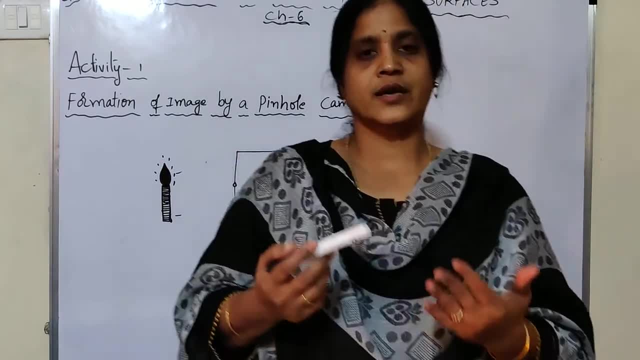 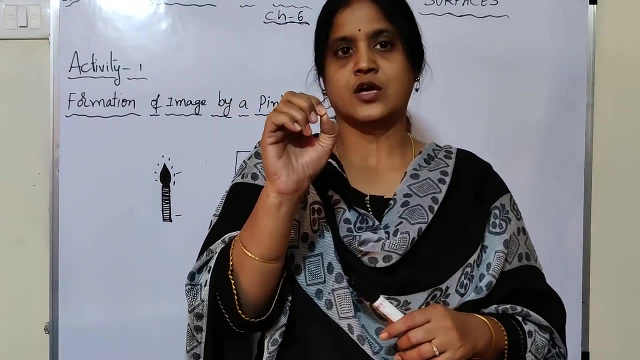 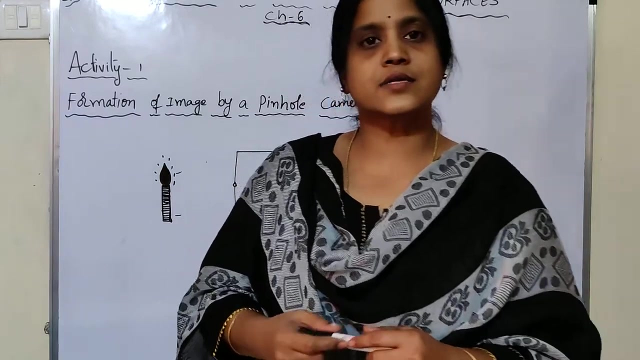 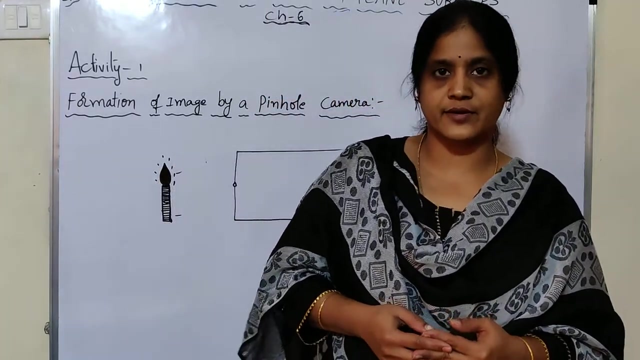 pinhole camera. without using the lens, we can capture the image on the screen. in the pinhole camera it has a small hole, so that hole acts as the lens, that the hole itself it acts as a lens, and this pinhole camera works on the principle of a rectilinear propagation of light. the spin. 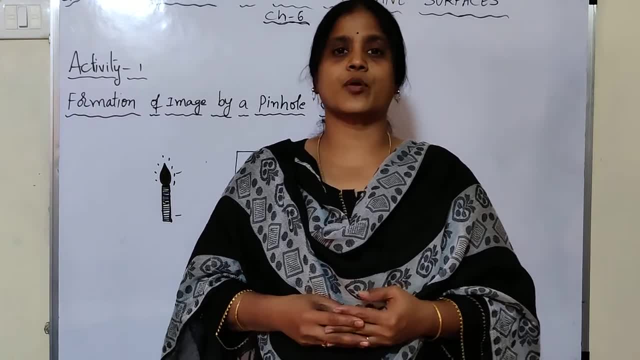 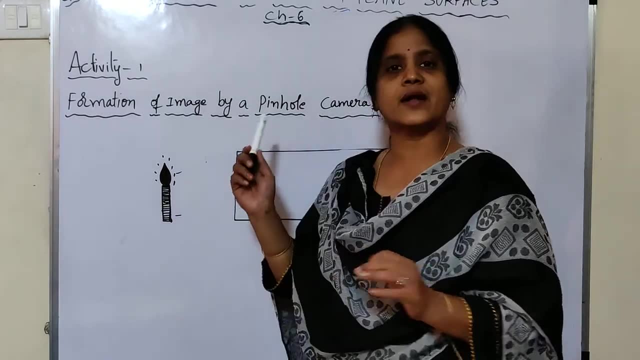 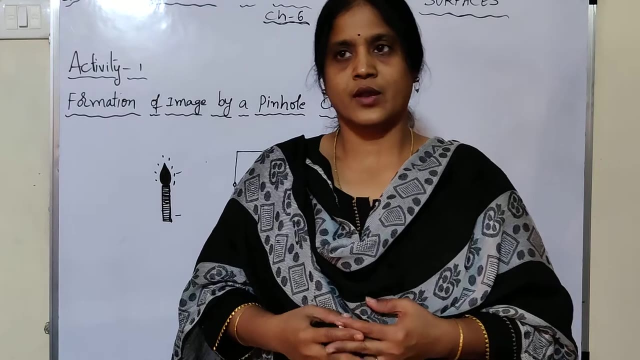 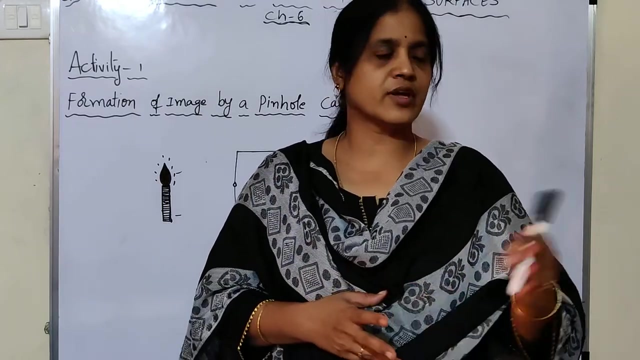 hole camera works on which principle? rectilinear propagation of light and the formation of image by the spin hole camera depends upon the size of the hole. size of the hole and for the preparation of this pinhole camera, just, you can take any box, cardboard boxes. we used to get package boxes, so you can take it and you have to. 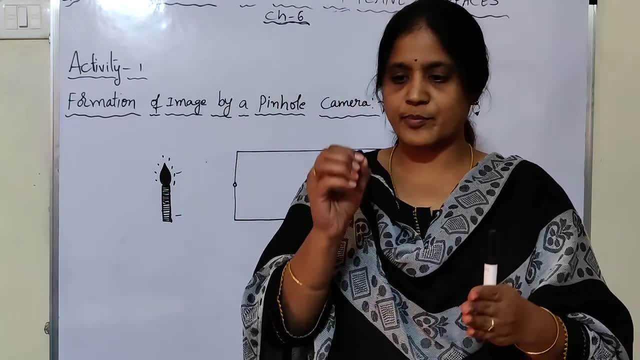 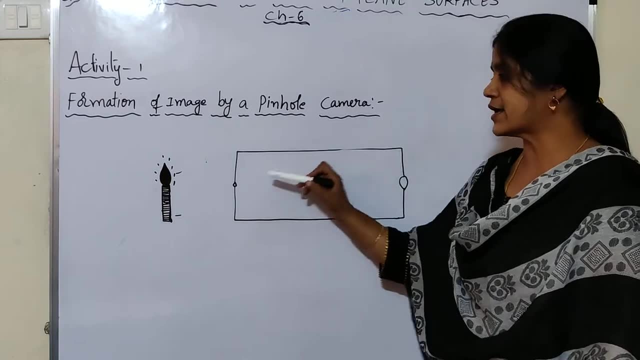 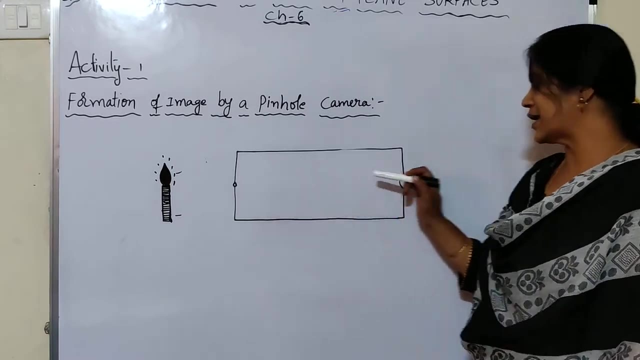 close it by a black paper. and if you make, just make a small hole at one. and here you see, take a one type of box, rectangular box, and at one face you make a small hole and exactly opposite to the hole, another end, and that's exactly opposite. 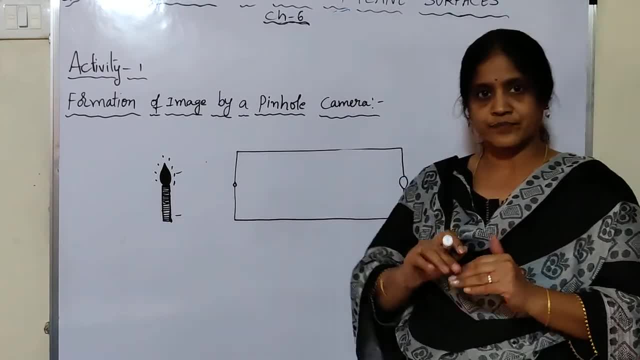 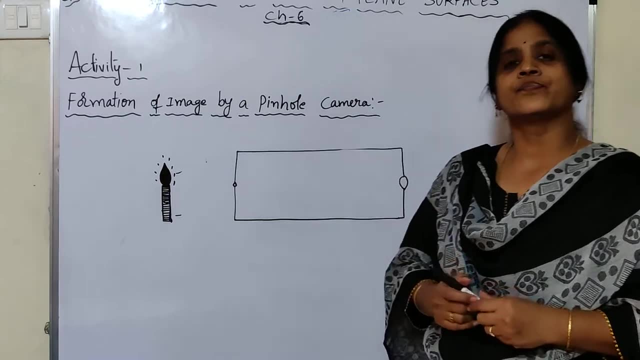 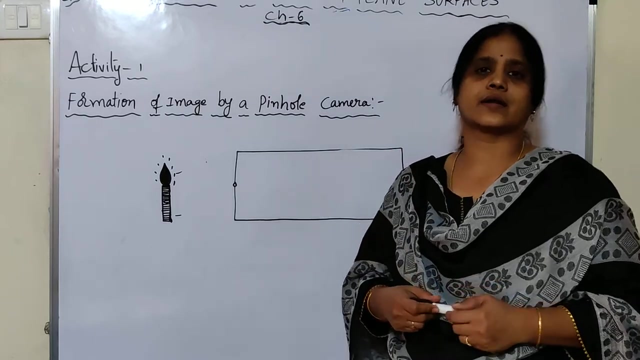 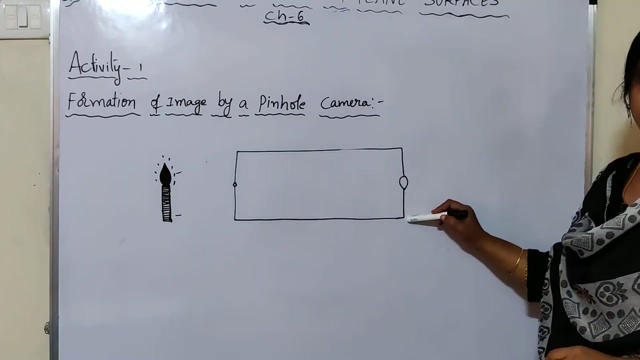 side. you have to cut the cardboard size paper that, whatever the paper, cardboard paper is covered that surface, you have to cut it and paste butter paper because you have to capture the image on that butter paper. this is the arrangement and you get the image. this is the butter paper. so you, you get the image on this butter paper. so the size: 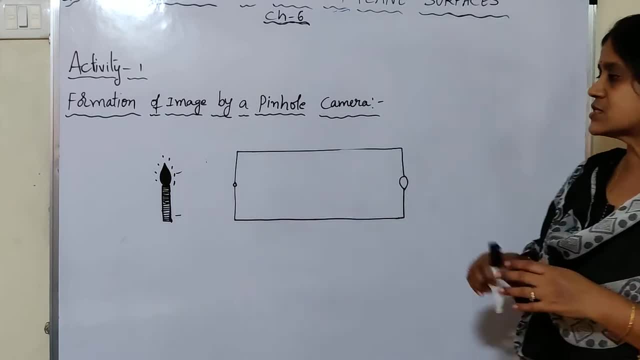 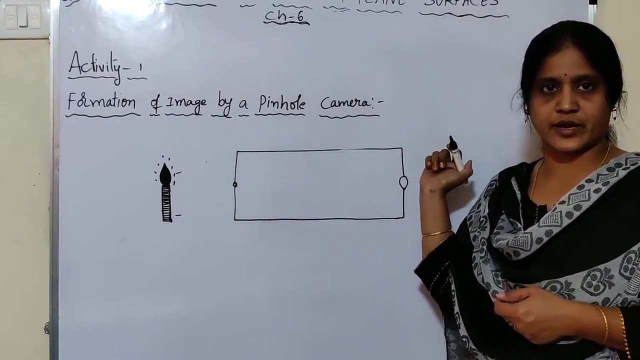 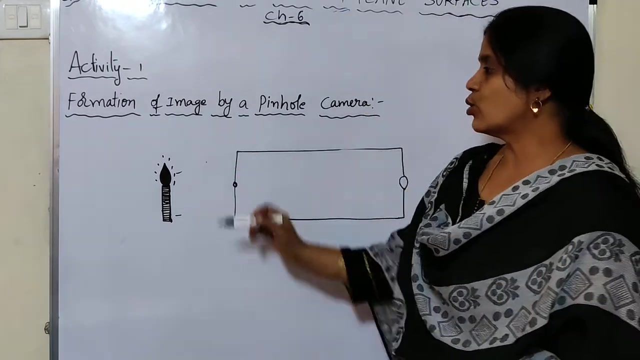 of the image formed by this pinhole camera depends on this size of the hole. to get the image on this screen, you have to take a source of light. so here, take one candle and light it, and when, light it from this flame. and here one more precaution we have to take it. 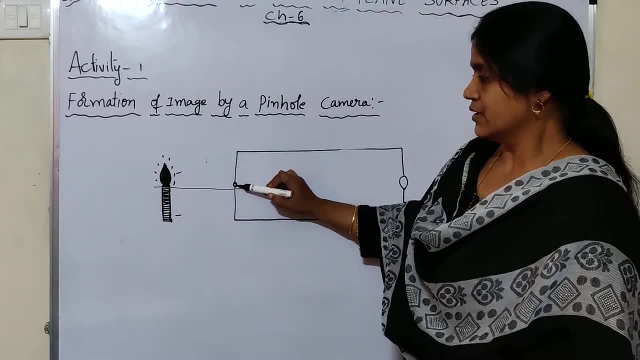 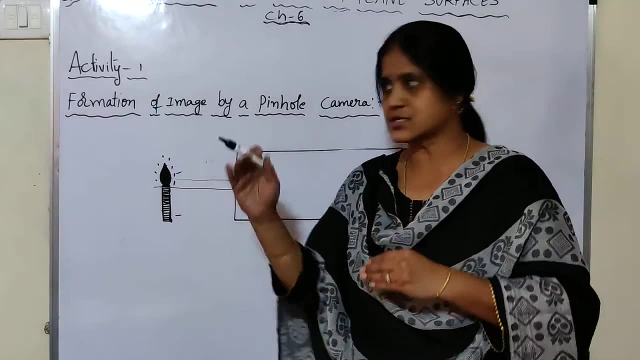 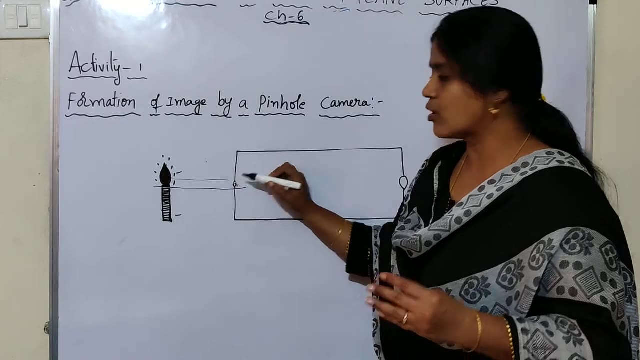 you see, the flame of the candle is exactly beside. I means these. these two should be in the strike length, like that. you have to arrange this candy. so when then, from this flame, when the hole is very small, few of the light rays. it emits the light in all the directions. 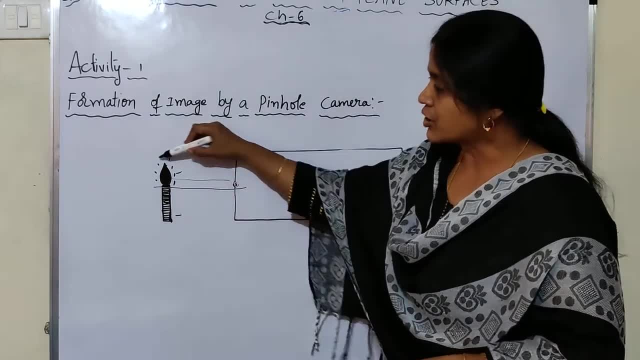 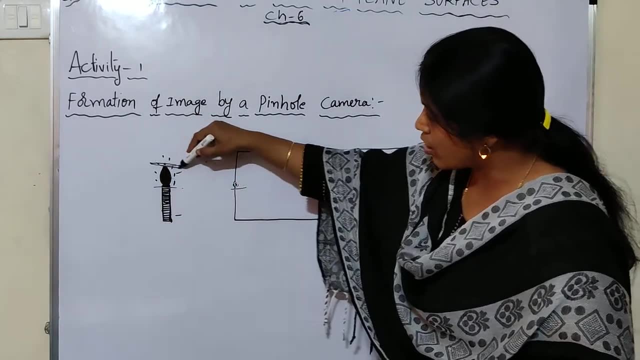 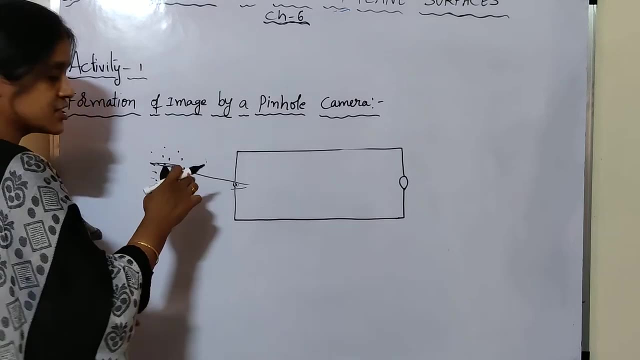 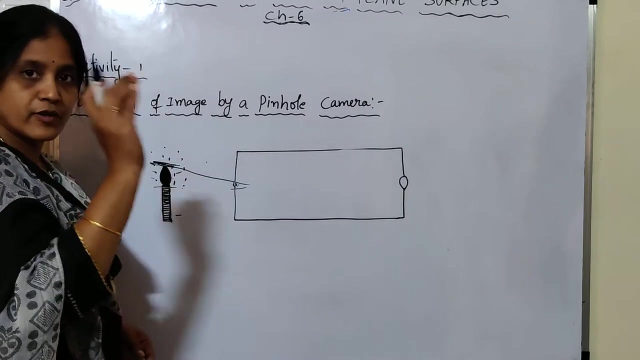 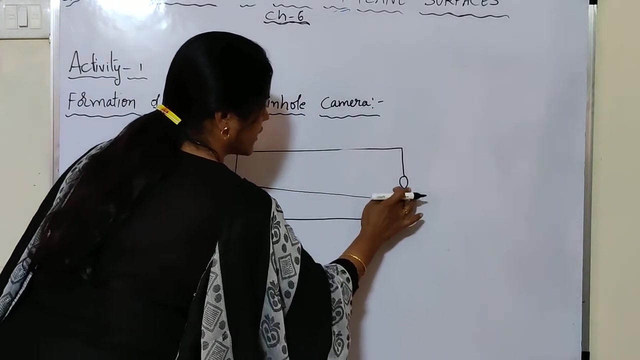 from that few of the light rays. from the top end of this flame these light rays they into this small hole. from that it emits light rays in all the directions, but out of that- only from the top of the flame- few of the light rays. that enters through this small hole and it falls on the screen. 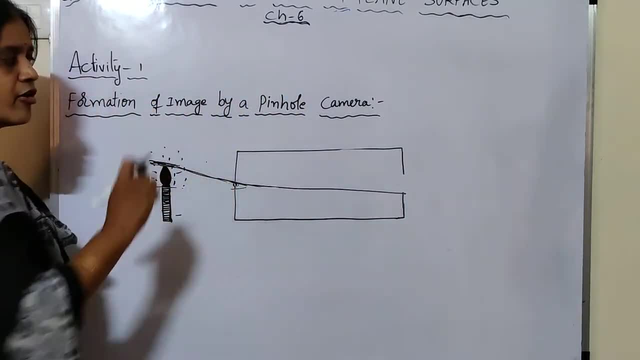 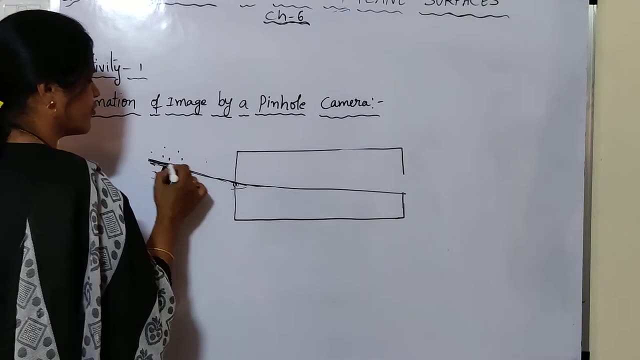 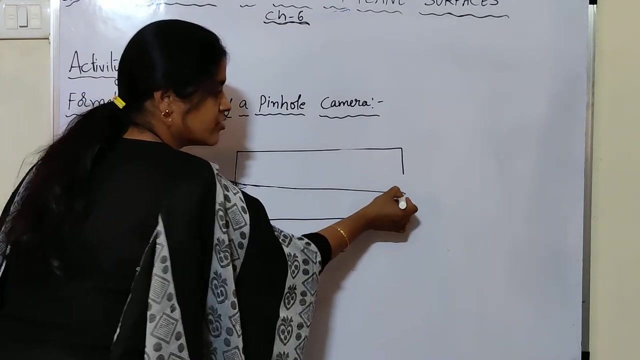 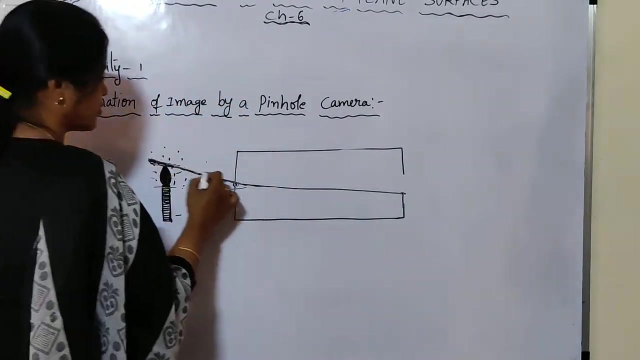 it falls on the screen here at the bottom and here a two or three or four, any rays from the top of the flame, all that travel and then the converts on the screen at one point. they converts on the screen at one point. all these rays, either two or three or four or whatever. maybe you take any rays, all that. 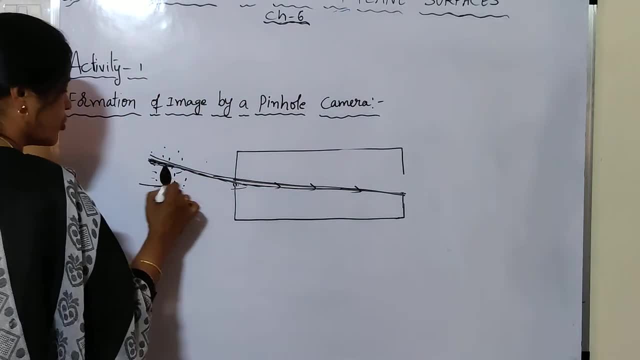 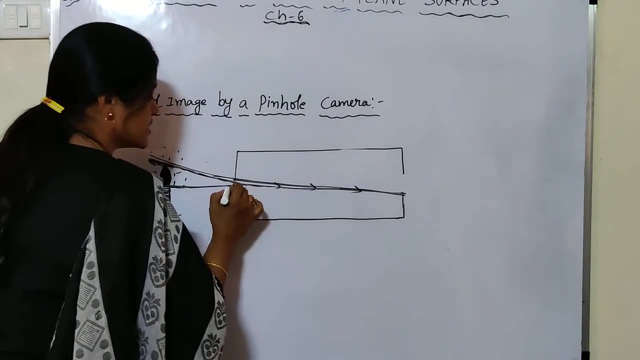 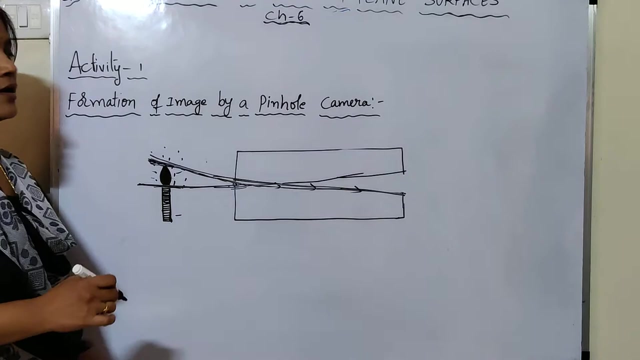 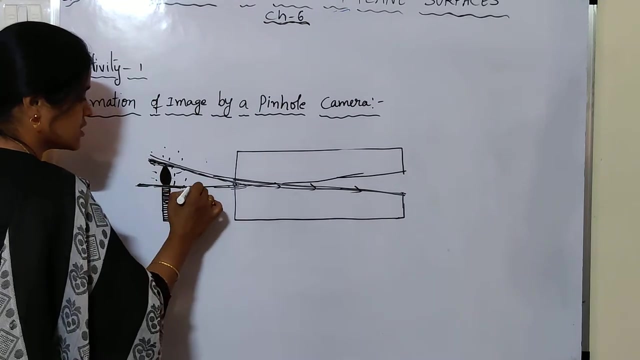 converse at one point now from the bottom of the flame and here also a few rays. they're passing through this small hole and they are. these rays will converse at the top end of the here at top, toward where they will converse from the bottom of these light rays they converse at the top of the screen here. 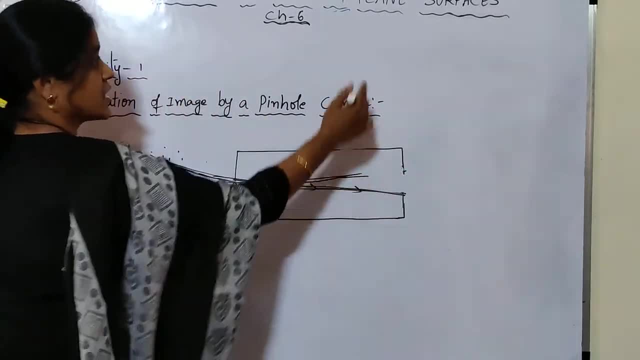 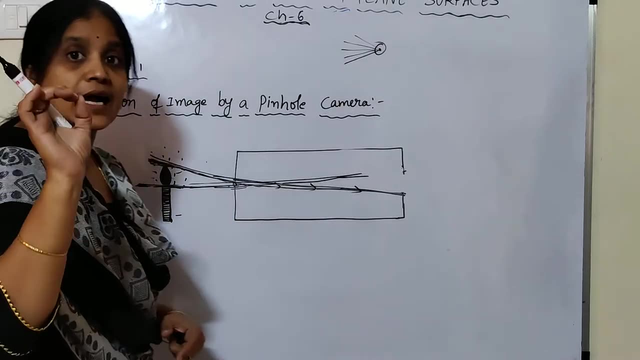 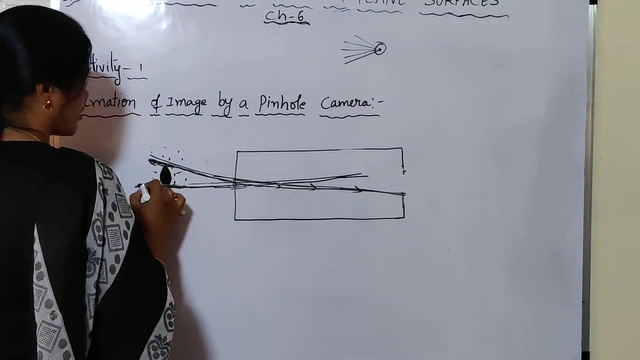 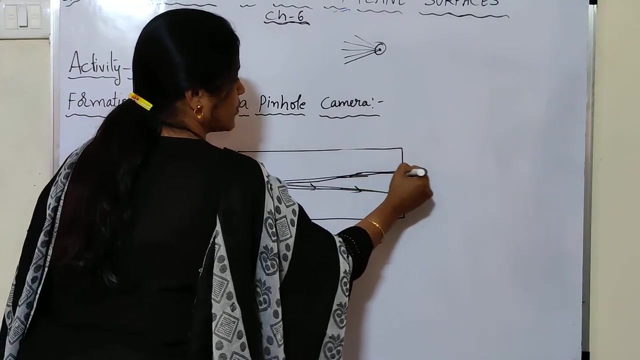 like this: all they will converge. converge means, from the different places, all the light rays, they will meet at one point. that will call it as convergence and this point we call it as converging point. so here, from the bottom of the flame, different rays, they all they converge, they will meet at one pointso. 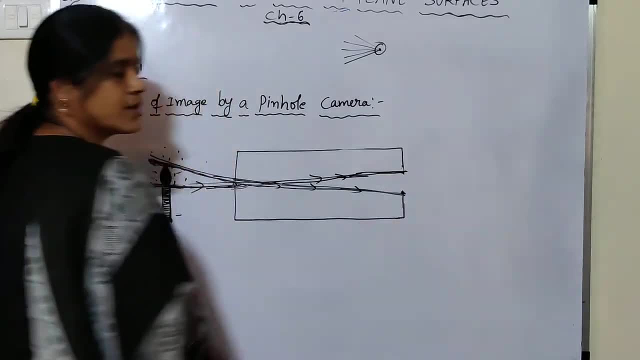 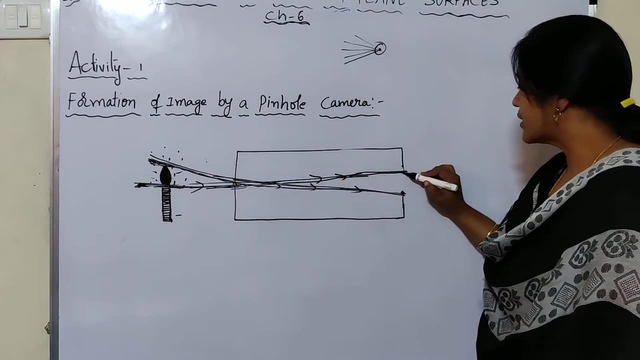 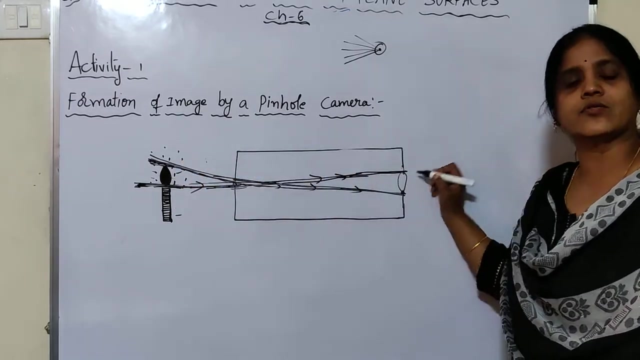 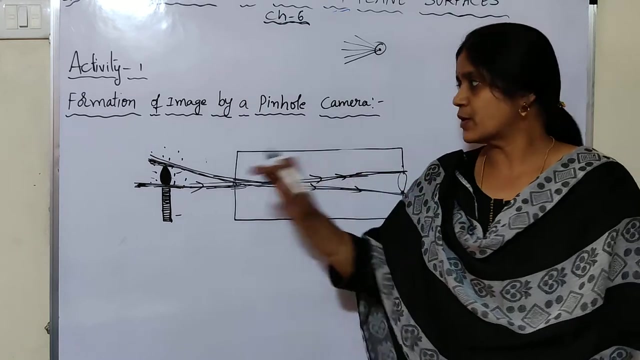 when they converge. we get the image. we get an image of this flame on this screen and it is exactly how you will get the size of the flame at the same size of image you will get on the screen and it is very sharp image. it is the exactly sharp image of this flame and you can get a clear image when you will. 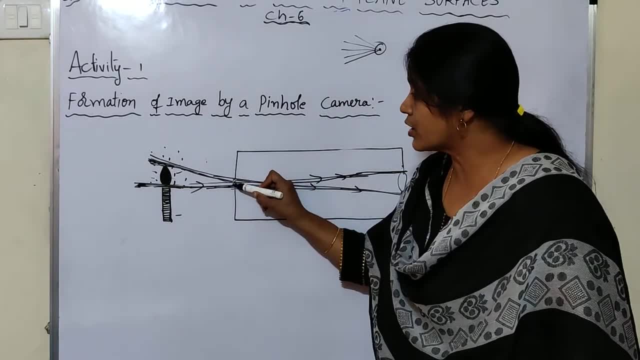 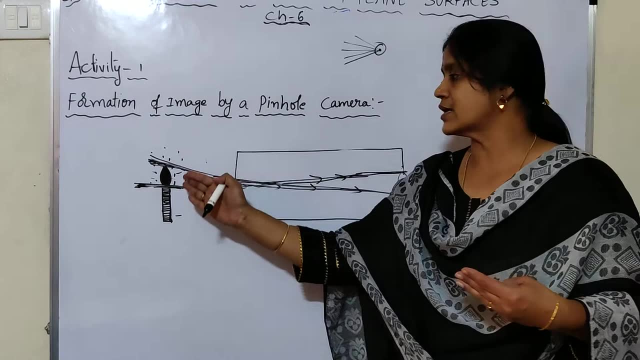 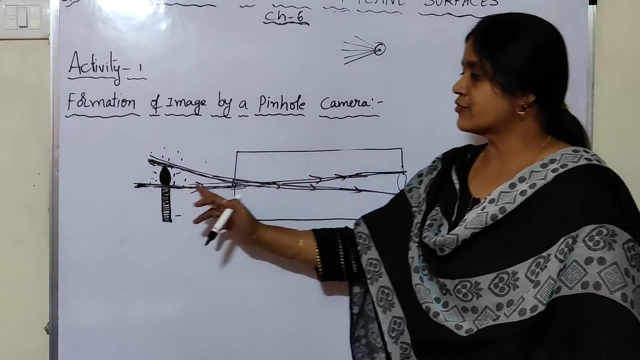 get a clear image when here and the pinhole camera, when the hole is very small and you can get the few light rays, they are passing from the top end of the flame passing and they converge at the bottom of the screen. i like that from the bottom of the flame these light rays passes through the 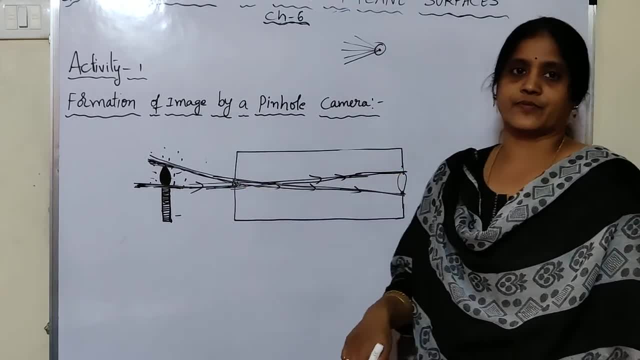 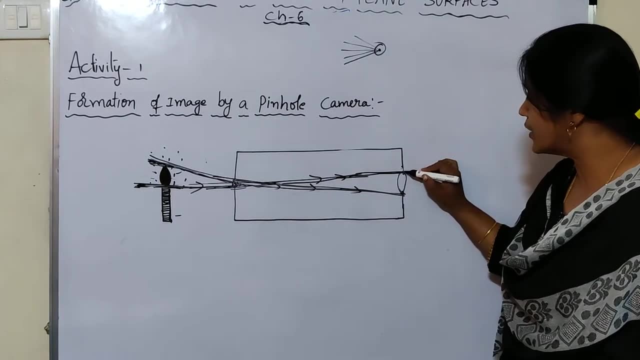 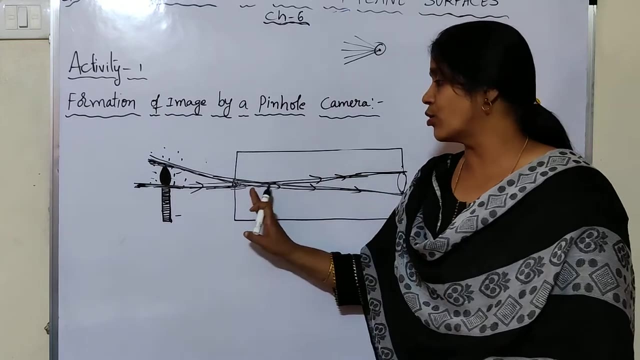 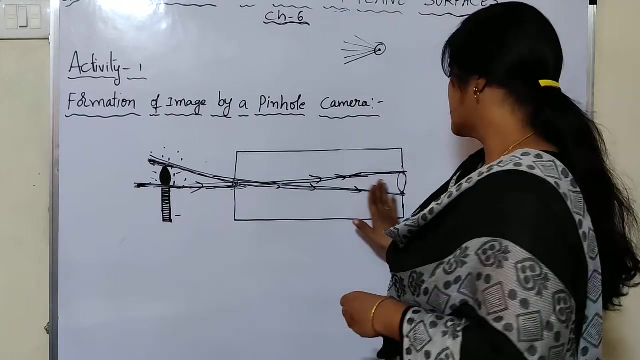 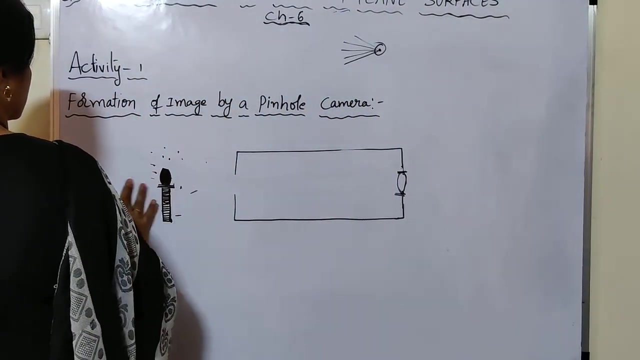 hole and they will converge at the top of the flames, top on the screen. so when the racer we get a sharp image on the screen. okay, suppose if there is a change in the size of the hole in the pinhole camera, then what type of image we get? what type of image we get, suppose, if i make like 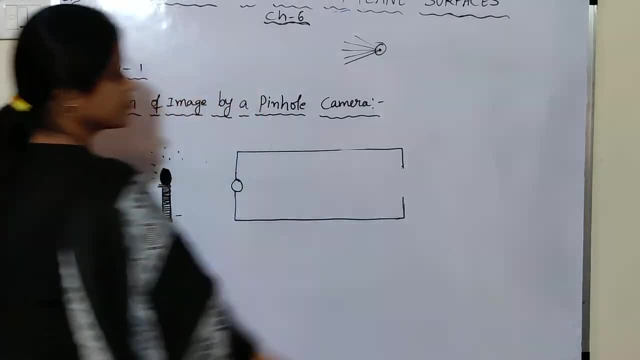 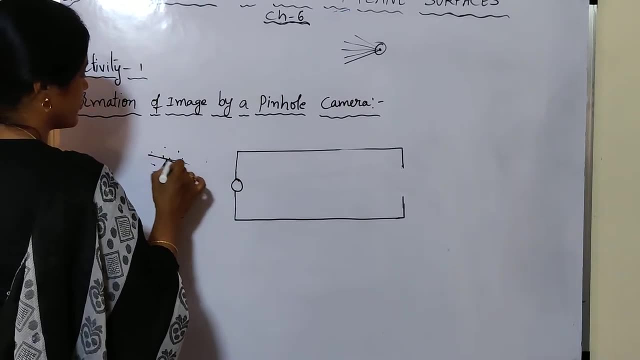 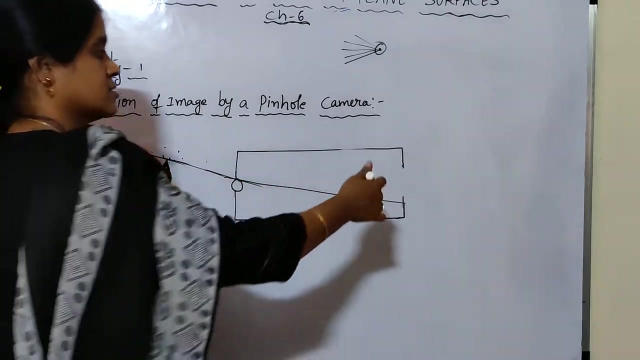 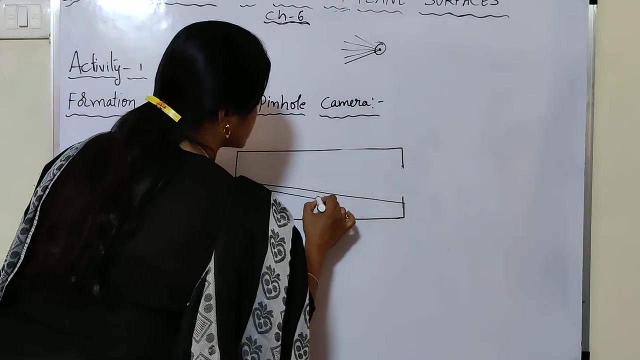 this big hole and what type of image we get, we'll see. this is the candle. so, as usual, from the top end of the flame, few of the light rays. they will pass through this hole and they meet on the screen at the bottom here. in the last case, when the hole is small, the light rays they will converge here. 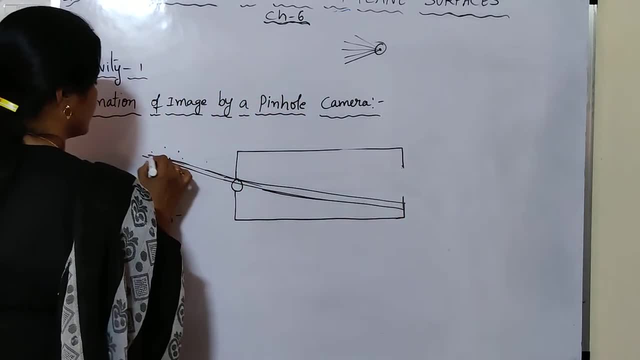 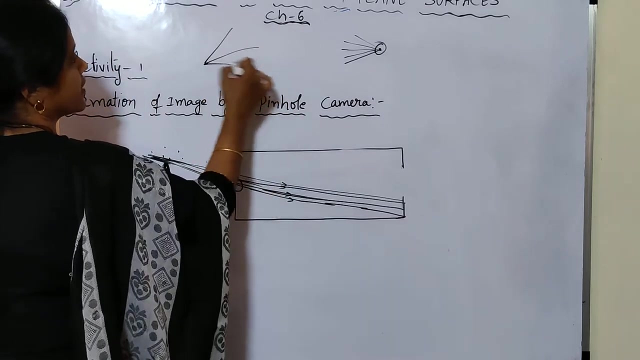 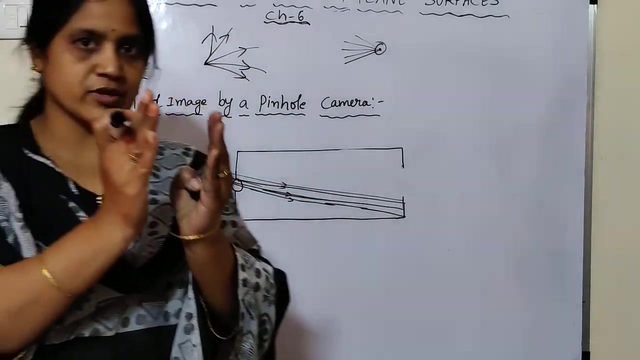 but here the light rays are diverse. from the top end of the flame, the light rays which are coming through the hole are diverging. they are diverging, so they are not meeting at one point. diverging means they are deviating in the different directions, so when they deviate they will not meet at one point. when the racer converges, then only we. 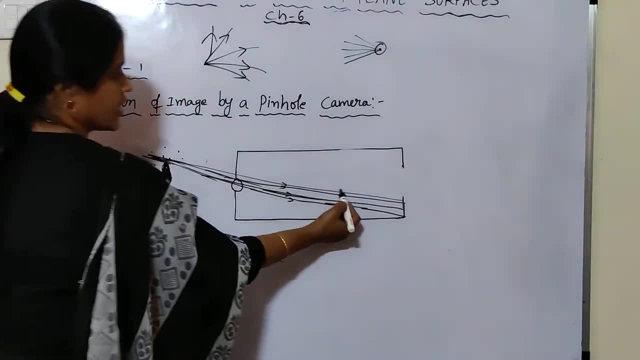 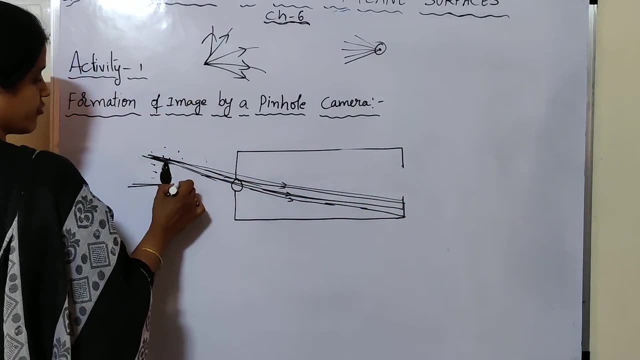 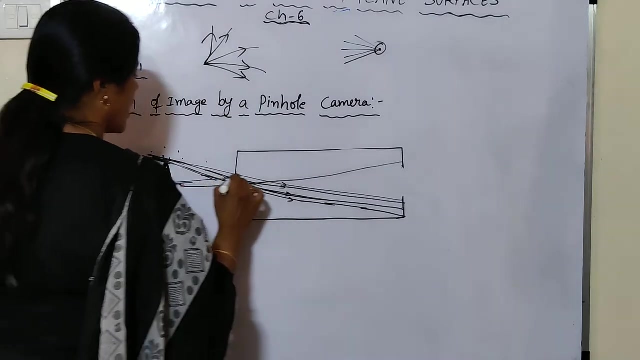 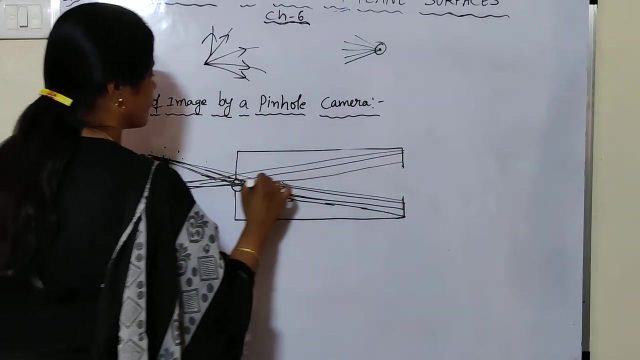 can get a clear image here. the light rays are diverging due to here at the bottom. you can observe like that you can if you see the bottom of the flame. from this, the light rays enters through this hole and falls on the top of the screen and these two light rays also diverges like this and they are not falling at one. 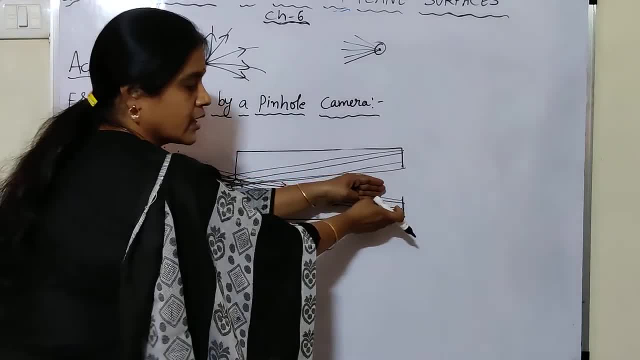 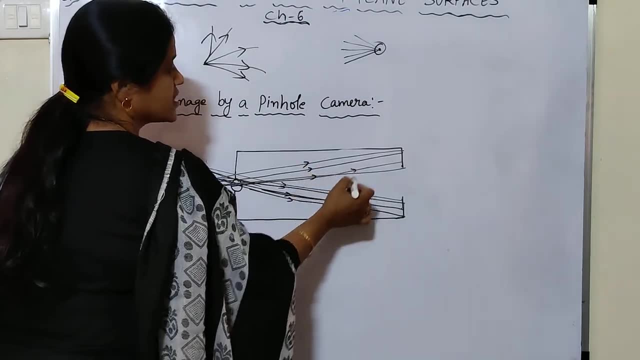 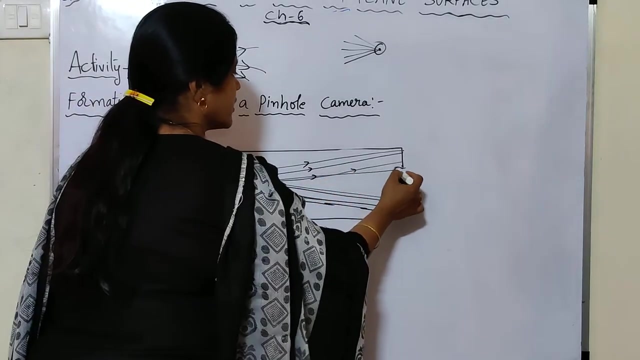 place all these light rays. they are not falling at one place. when the light rays falls at one place, we get a sharp image, but here all are diverging. due to this, the due to this reason. you can get the image on the screen. you can get a image on the screen, but that image is not clear. 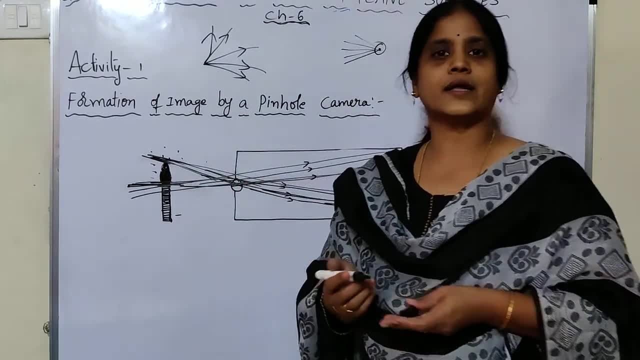 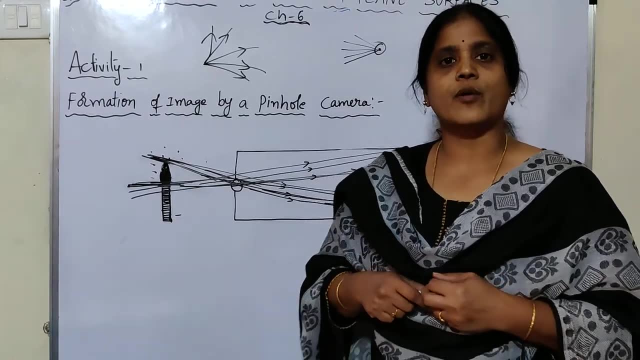 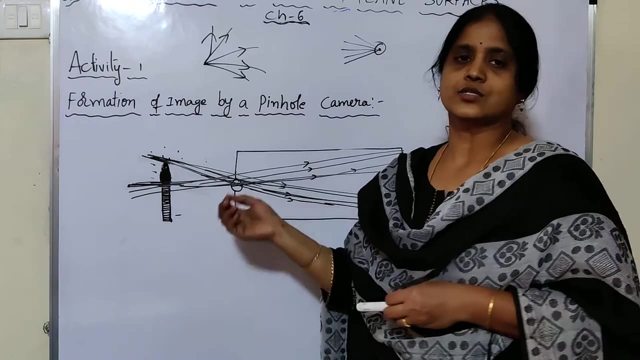 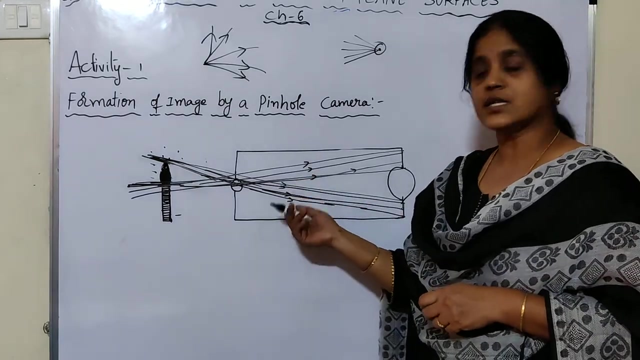 you can get a blurred image. you can get a blurred image and two years back they asked one question: draw a ray diagram for the formation of image by a pinhole camera when the size of the hole is big. so this is important for two marks: drawing the ray diagrams. arrows are very important. these arrows represents the. 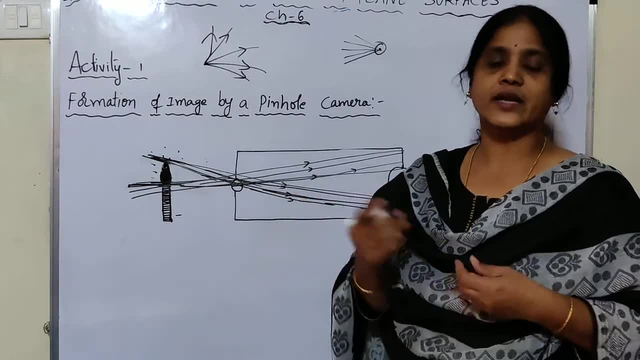 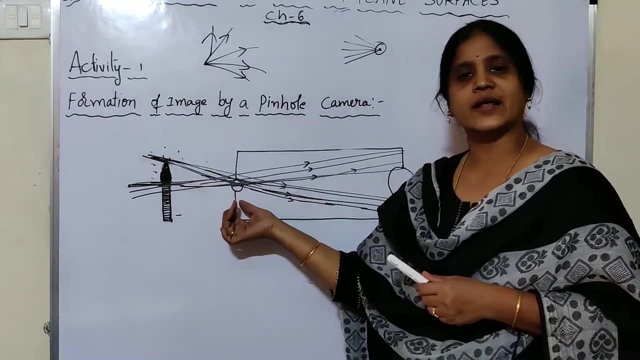 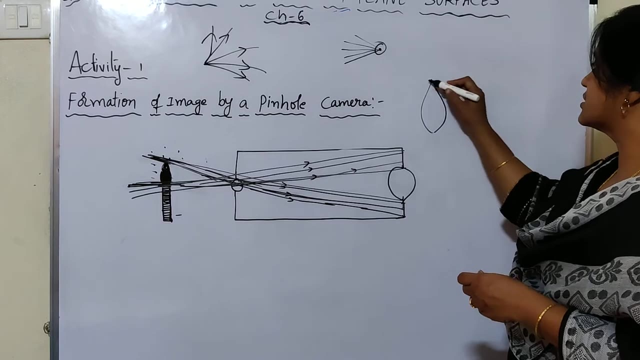 towards which direction the light rays are trap. it indicates the direction of the light rays and the image formed by the spin hole camera is always invert image. suppose the flame is like this: you will get the reverse- this top, you will get the bottom and the bottom, you will get the top and you will get the image. 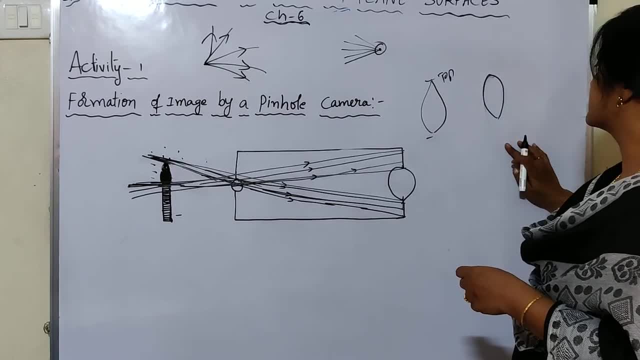 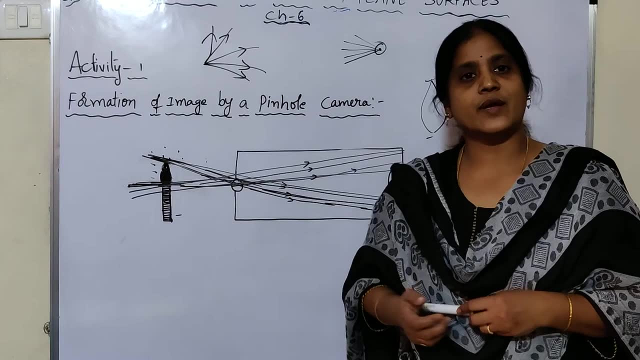 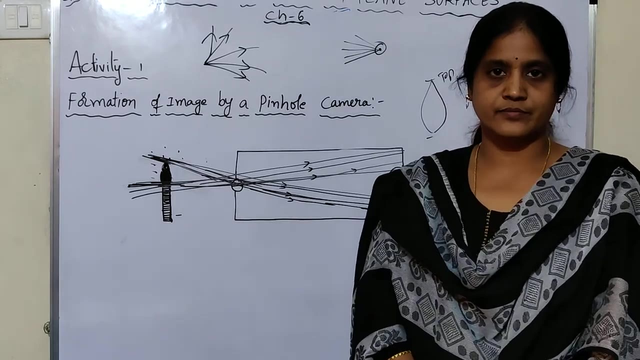 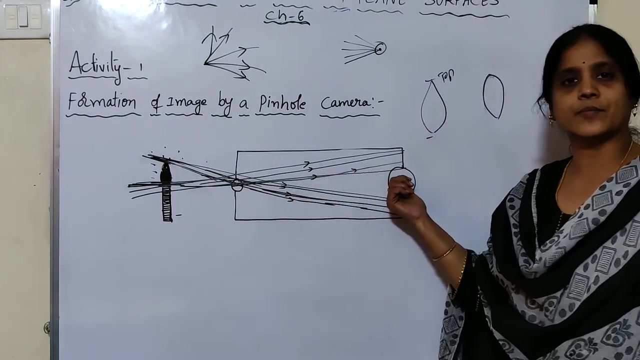 like this and you will get the image like this. so always these images are inverted images and these inverted images are real images. so this is about pinhole camera, thank you. and one more thing see here: if you make one hole, you can get one image. for example, if you make instead of one hole on this face, if 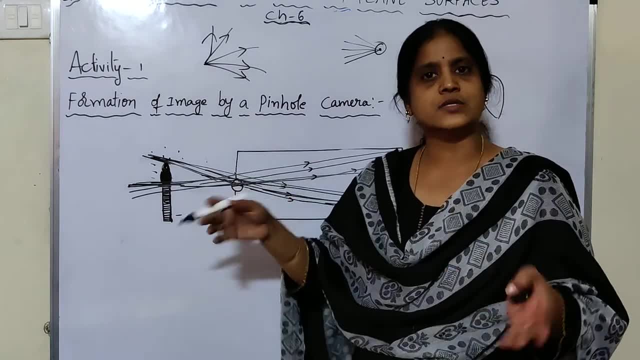 you make one hole on this face, if you make one hole on this face, if you make you make one hole on this face, if you make one hole on this face, if you make more than two holes, our five holes and ten holes like this, if you make or